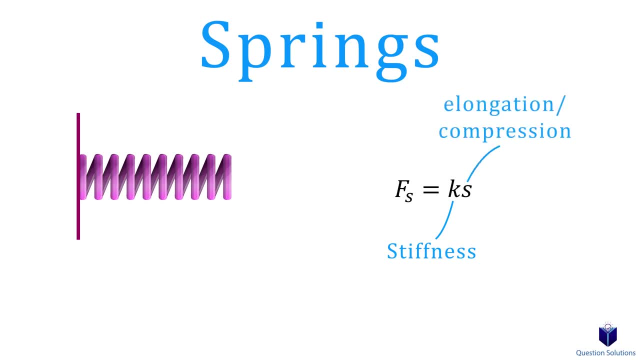 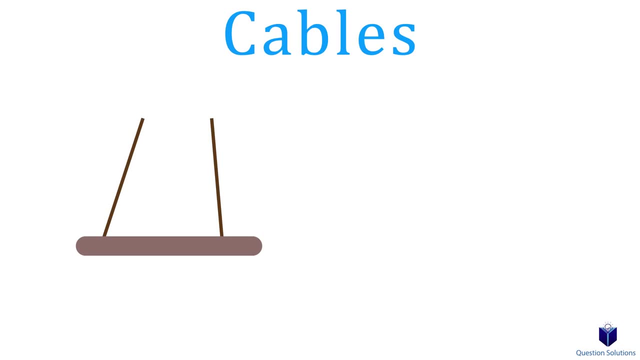 K is the stiffness of the spring and S is the elongation or compression. Next, we need to discuss cables. A cable can only support a tension or a pulling force. Remember you can't push on a rope. This force will always act in the direction of the cable. If we have a 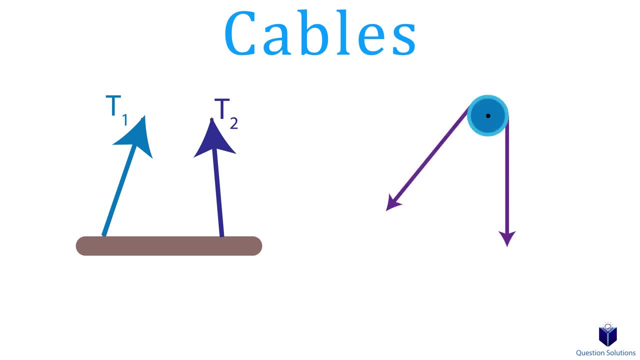 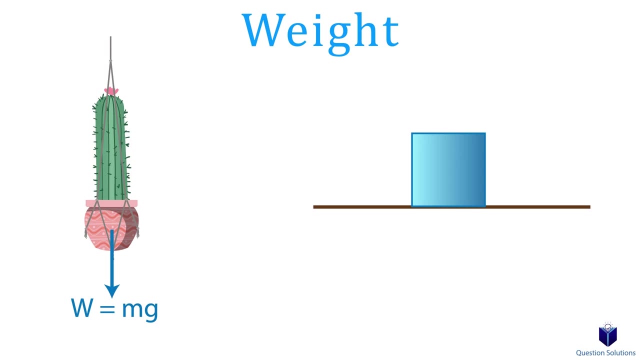 cable going through a pulley, the tension throughout the whole cable will be the same. Lastly, objects have a weight, and that's simply the mass of the object times the acceleration due to gravity, which is 9.81 meters per second squared, or 32.2 feet per second squared Weight. 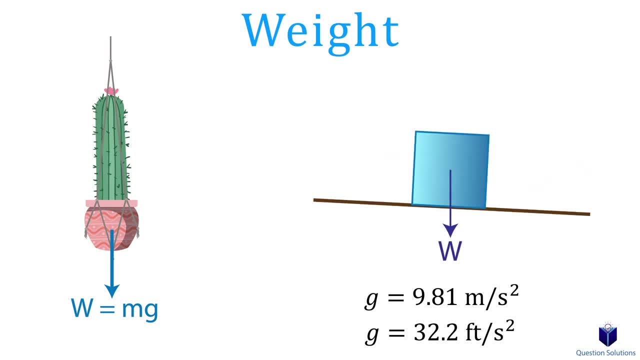 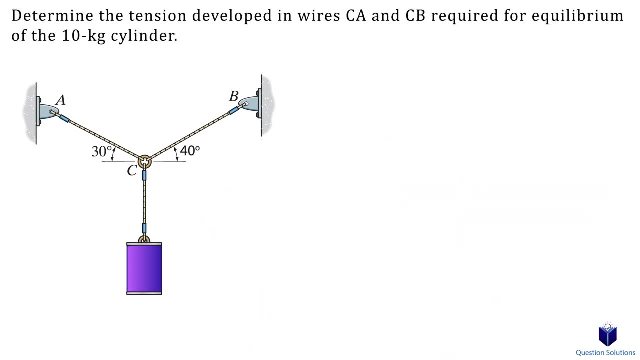 is always straight down, even if an object is on an inclined plane. Now let's move on to some examples to see how we can solve for unknown forces. Let's take a look at this problem where we have a cylinder in equilibrium. We need to figure out the tension developed in the wires CA and CB. 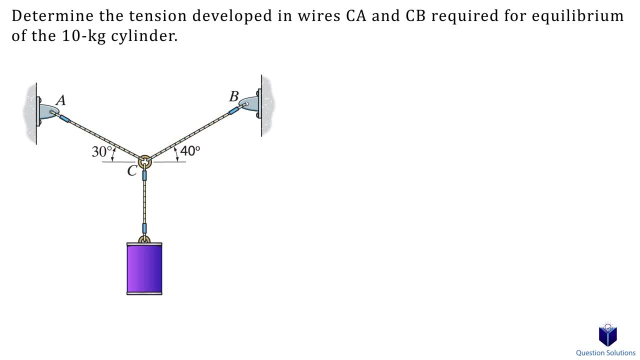 The first step is to pick our point where we will write out equations of equilibrium. For that we will pick point C. Now we draw our coordinate system, So we have the x-axis and the y-axis. Next we can draw our forces. We have a force in the cable CA, a force in cable CB. 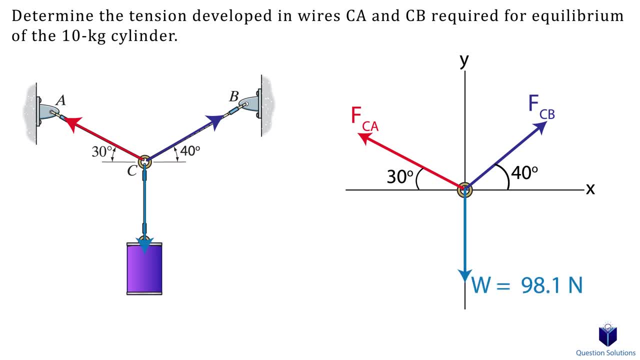 and we have the weight of the object downwards. The weight is the mass of the object times the acceleration due to gravity. This is the mass of the object times the acceleration due to gravity. So that would be 98.1 newtons. Now we can draw the components of each force. 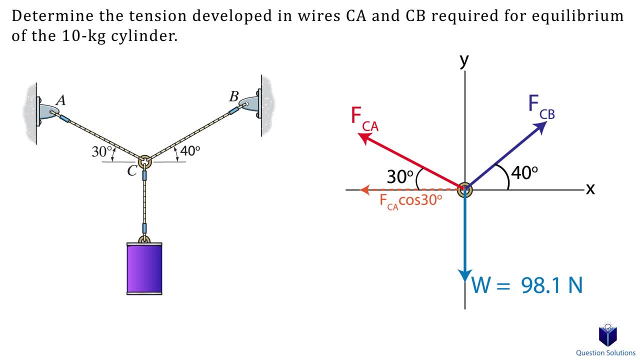 Let's focus on force CA. We have the x component, which can be found using cosine, and the y component, which can be found using sine. Now for force CB. If this is unfamiliar to you, please check the description for vector addition of coplanar forces, where I explain how. 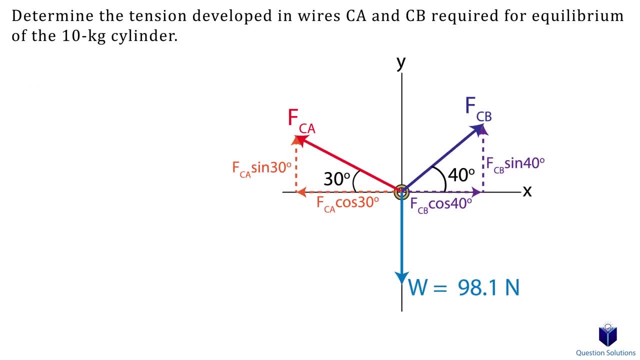 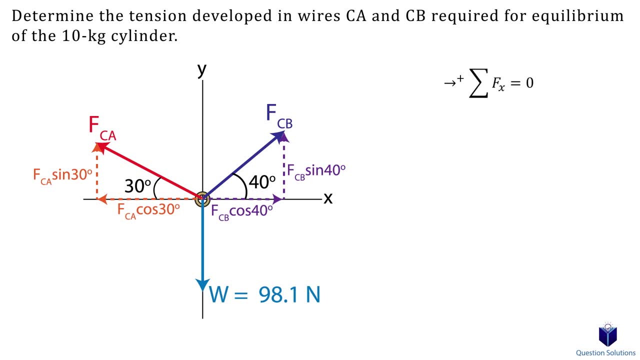 to break forces into components, step by step. It is time for us to write our equations of equilibrium. First, for x-axis forces, We will assume right is positive. So we're just looking for any force that lies on the x-axis. We see two forces. We have the x components of forces, CA and CB. 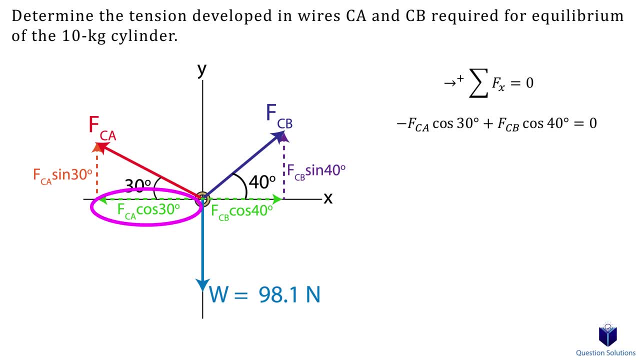 Notice that the x component of force CA is facing to the left, so it'll be negative. Next we look at y-axis forces. We will assume up to be positive. There are three forces to consider. We have the y components of force, CA and CB. 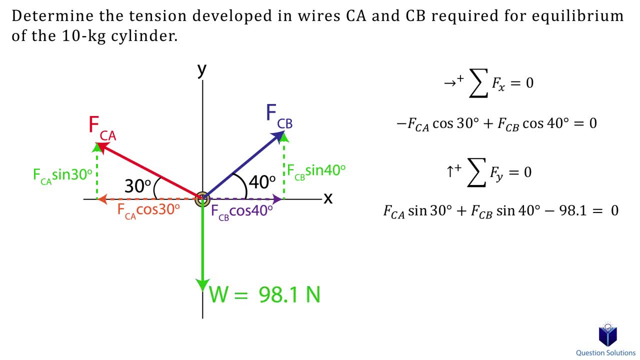 and we have the weight, which is straight down. Since the weight is downwards, it'll be negative. We now have two equations with two unknowns. You can solve them any way you like. So these are the tensions in the cables to hold the 10 kg cylinder in equilibrium. 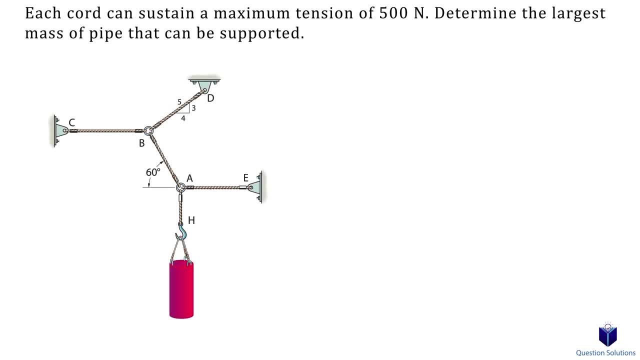 Let's take a look at this problem, where we have multiple points to consider In this question. we're told that each cable can support a maximum tension of 500 newtons, and we need to find the largest mass of the pipe that can be supported. 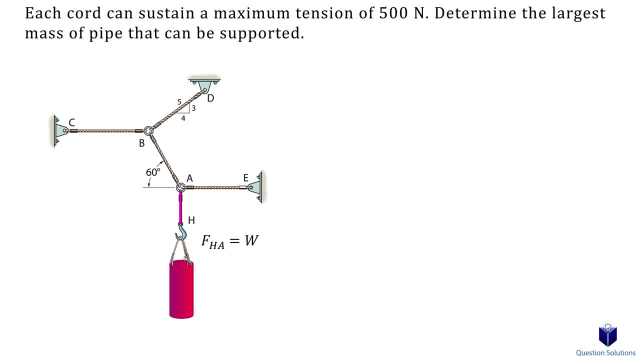 So straight away we know that the tension of cord HA would be equal to the weight of the pipe. Now, leaving that to the side, we can look at point A and draw a free body diagram. We have the force of cable HA downwards, force of cable AE to the right. 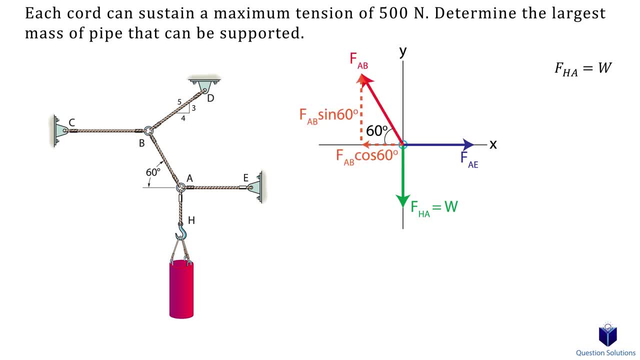 and we have the x and y components of force BA. So let's write our equations of equilibrium, First for the x-axis forces, and we will assume right to be positive. Next we look at y-axis forces, We will assume up to be positive. Instead of writing force AH, we can write the weight, since 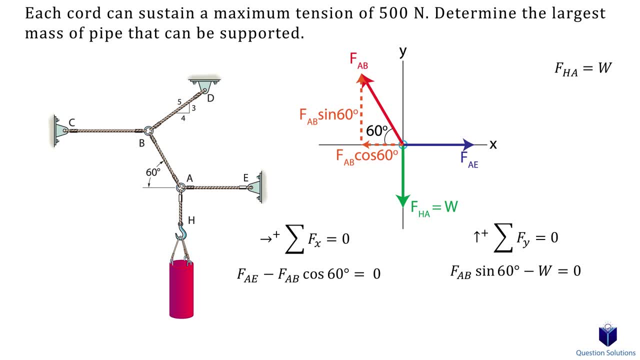 they're equal. Let's isolate this equation for force AB. Now we can use this value and plug it into our previous equation to isolate that one for force AE. You will see at the end why we do this. Let's set those equations to the side and draw a free body diagram for point B. 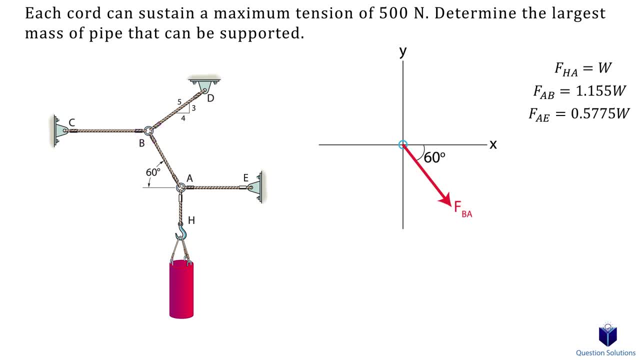 So we have force BA. that now points downwards, we have force BD and we have force BC. We can also draw the components of force BA like this: The components of force BD can be found using the ratio triangle given to us. Now we will write our equations of equilibrium. First, for x-axis forces. 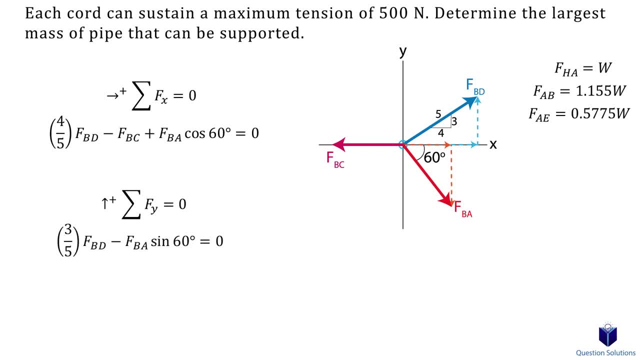 Next, y-axis forces. Now, if we look at the equations we came up with before, we see that we already wrote force AB in terms of weight, so we can actually plug that value in for force BA. Let's isolate for force BA. 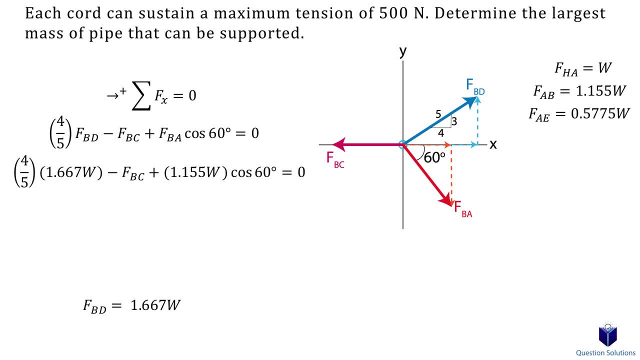 Now we can plug this value into the previous equation to write force BC in terms of weight. So the reason why we wrote every force in terms of one weight is to compare which cable would carry the largest force. If we look at the four values we have, 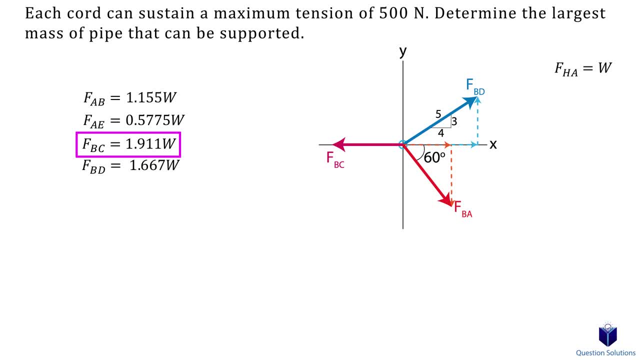 we see that force BC would have the largest tension, since it's the biggest number. So all we have to do is figure out what weight would cause force BD to equal 500 newtons. Let's solve for the weight Now. if we divide the weight by the acceleration due to gravity, 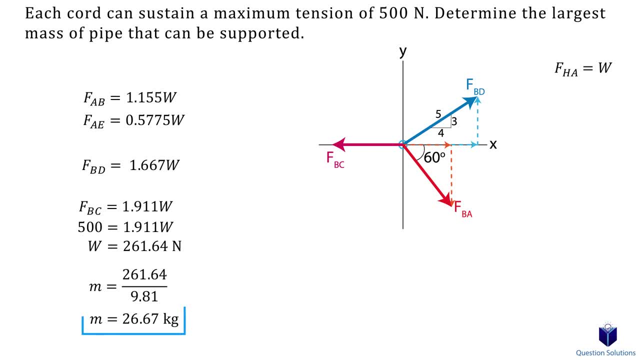 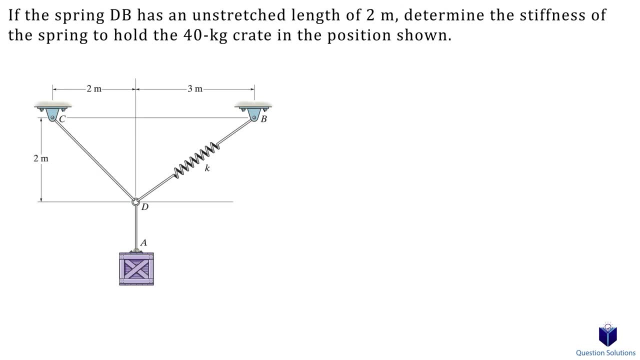 we get the mass. So the maximum mass of the pipe that can be supported is 26.67 kg. Let's take a look at a question involving springs. Here we need to find the stiffness of the spring to hold the crate in the position shown Before we draw a free body diagram. 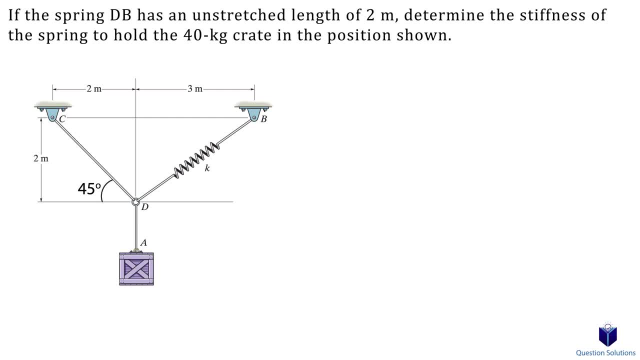 let's quickly calculate the angles. This angle can be found using tan inverse. Now for the other angle. Okay, now we will draw the free body diagram about point D. We have the force in spring DC, the force in spring DB and we have the weight of the crate. 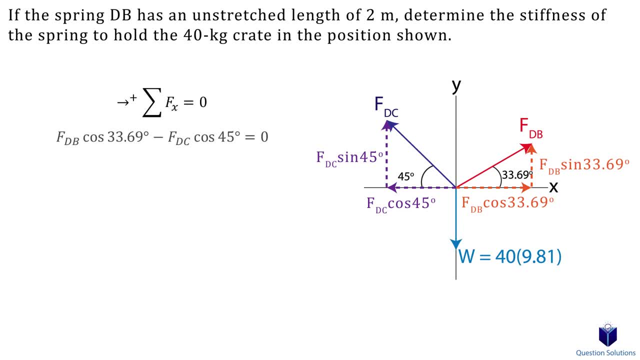 Now we can write our equations of equilibrium. Let's start with the x-axis forces. So we have the two x components of our cable and spring. Next we can write an equation for the y-axis forces. We have the two y components plus the weight, which is straight down. 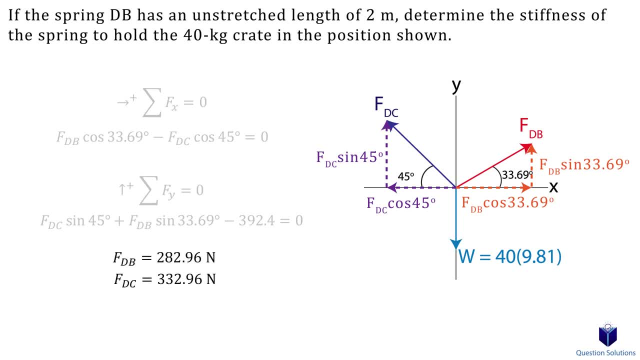 Now we have two equations with two unknowns. Let's solve them. So we figured out the force in the spring. The question tells us that the unstraightening force of the spring is the force of the spring. The length of the spring is 2 meters. Let's figure out the length of the spring after it was stretched. 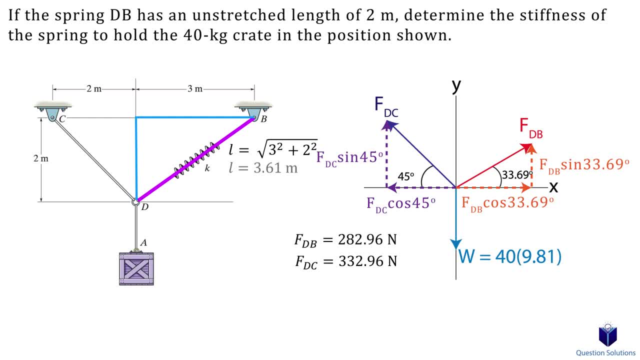 We can use the Pythagorean theorem for that. This tells us the current length of the spring. Let's subtract the initial length from this value to figure out how much it stretched. So the spring stretched 1.61 meters after the crate was hung. 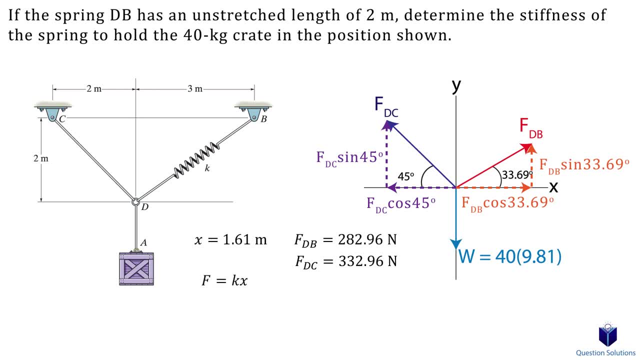 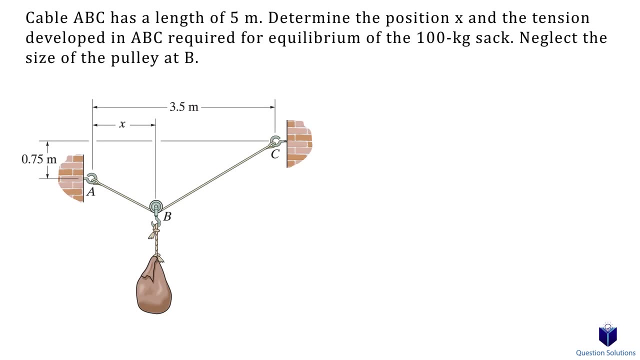 Now we can use Hooke's law to figure out the stiffness. The force is what we found before, so that's the force. in spring DB, The x-value is the length the spring stretched. Let's solve, and that's it. Let's take a look at one last example. This is the type of question that involves geometry. 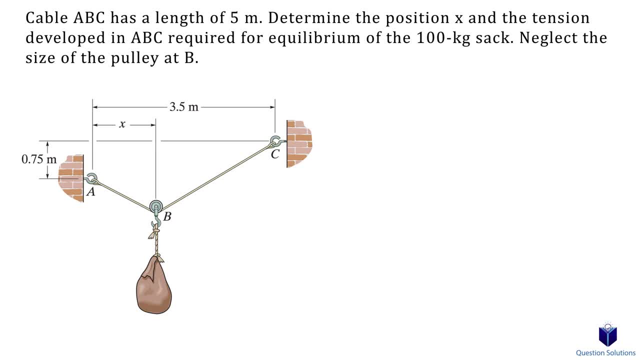 more so than the usual In this question. we need to find the x-value and the tension in the single cable required for equilibrium. So if we draw a free body diagram of point B, the forces that goes both ways can be represented the same, since it's a single cable. In other, 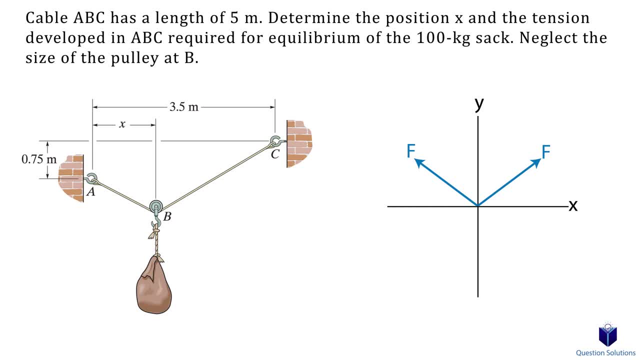 words, the tension in the cable is the same throughout the whole length. Now there are two that are created, and both of these angles would be the same as well. Lastly, we have the weight of the 100 kg sack. Let's write an equation of equilibrium for the. 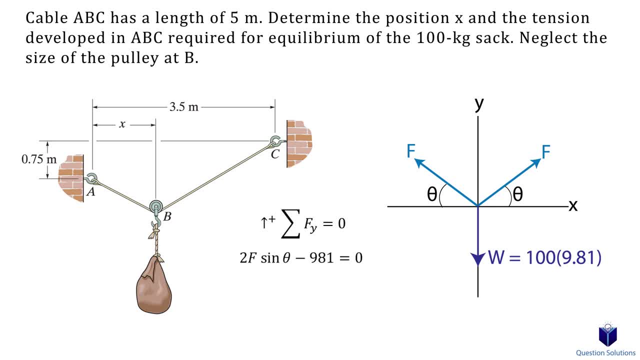 y-axis forces, We will pick up to be positive. Writing an equation of equilibrium for the x-axis forces won't help us, since it'll just equal zero, So instead we need to look at the geometry of the problem. Let's draw this diagram separately. Notice how these two angles 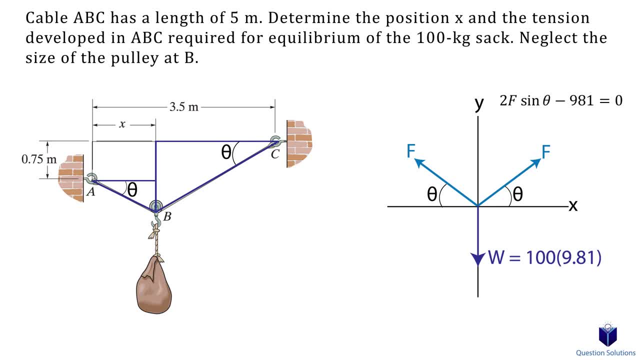 are the same as the angles on our free body diagram. This is because these are alternate interior angles. Now the total length of the cable is 5 meters. So that means if we add up the two hypotenuses of the triangles we have here, they must equal 5 meters, Since both are right. 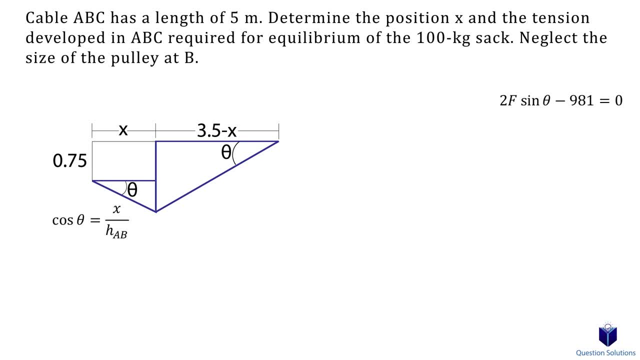 angle triangles. we can use cosine to write it out. For the small triangle we can say: the cosine of the angle is equal to the hypotenuse of the triangle divided by length x. Let's isolate it for the hypotenuse. Next, the big triangle. 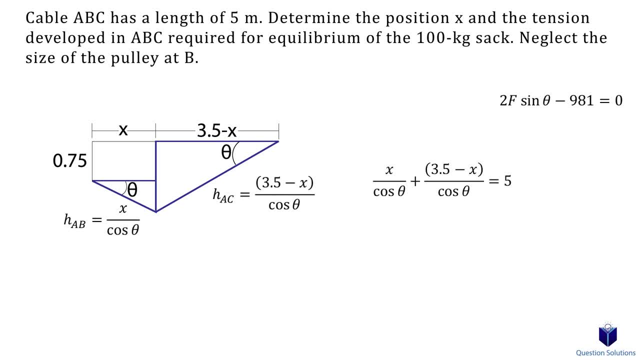 Now both of these hypotenuses added together must equal 5 meters. Let's simplify. Notice how the two x's cancel each other out. so we can solve for theta. Now we need to figure out the x-value. To do that, we need one more equation For that. 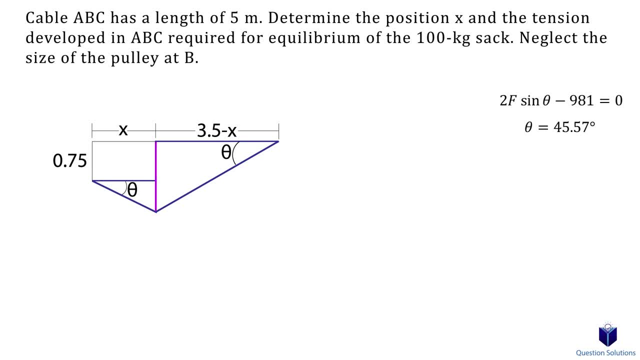 we will look at the opposite lengths in our triangle. Let's label that y From the x-axis. you can see this triangle here as well. If that is the objective of this small triangle, we can write tan like this: So remember it is opposite over adjacent. Let's isolate it for y. 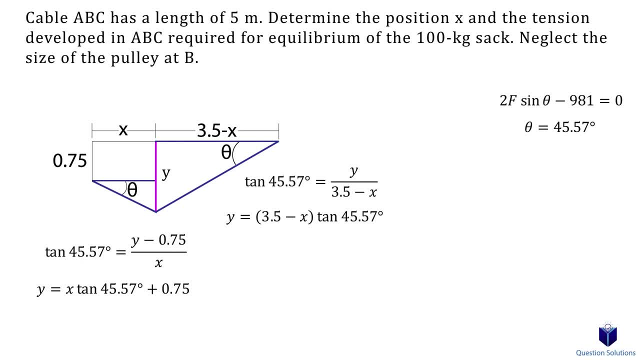 Next, from the side of the big triangle, we can write tan like this: Let's isolate this for y. Now we can plug one equation into the other. Let's solve for x. Now we can use the angle we found before in our forced equation to figure out the tension in the cable. Those are our answers, That 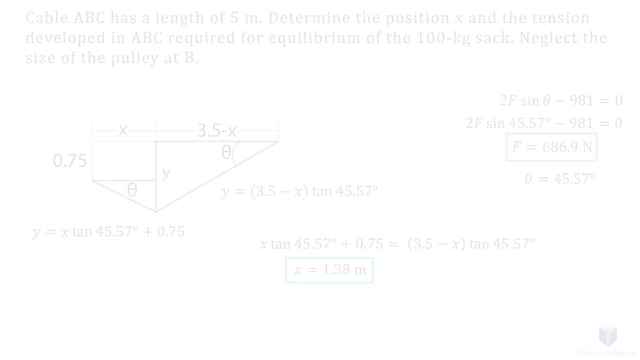 should cover the types of problems you will face when solving for those angles that are less than 1.5 meters. when it comes to 2D equilibrium, In the next video we will go over how to solve three-dimensional equilibrium problems. Thanks for watching and best of luck with your studies.